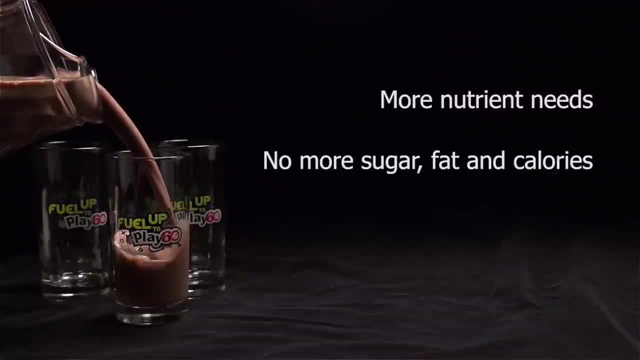 meet more of their nutrient needs, do not consume more added sugar, fat and calories, and are not heavier than non-milk drinkers. When it comes to flavored milk, it's only a small amount of added sugar compared to other beverages. Kids, why do you like to drink chocolate milk? I like drinking it in the morning. 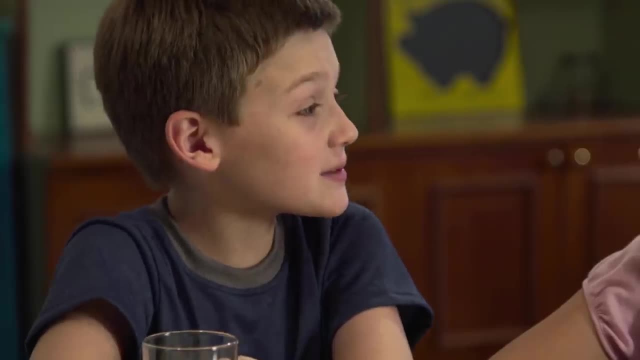 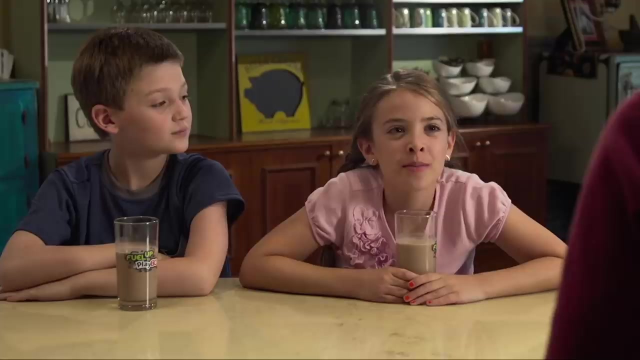 with my breakfast because you always say it fills me up for school And it makes me feel like I have a superpower. I like it because it tastes good, But my mom told me it helps me build up strong bones and I want to be big and strong. 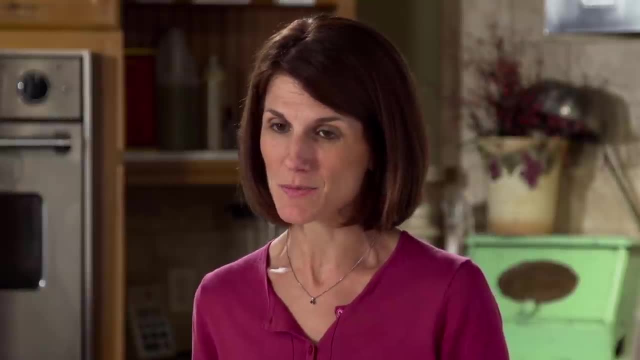 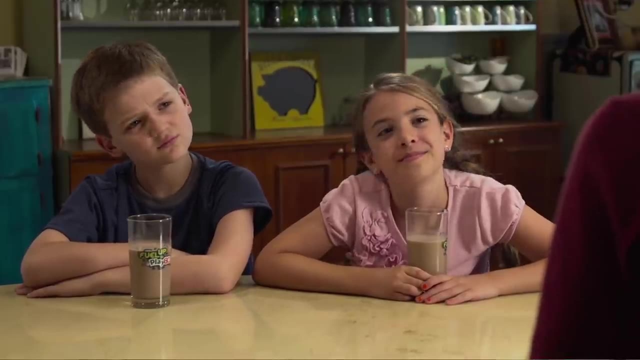 when I grow up. Well, I like it because it's affordable and it gives me peace of mind. A glass of milk only costs about 25 cents per glass, And when I give it to you and your friends, I know you're drinking something healthy, especially. 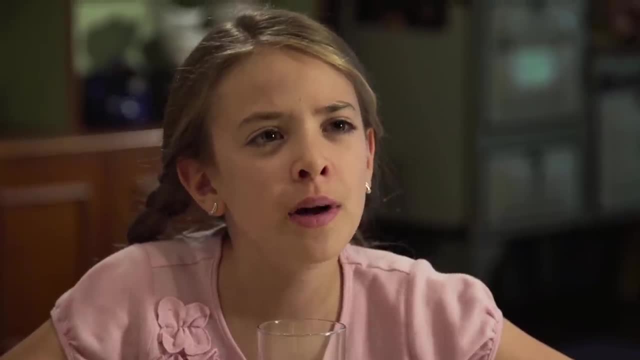 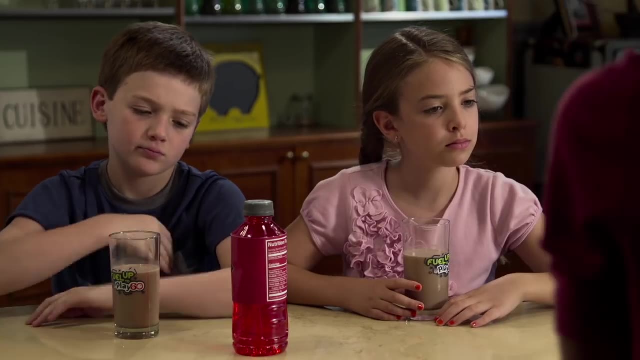 compared to other beverage choices. So you're saying that drinking chocolate milk is better than drinking a sports drink or soda? Yes, Here let me show you: Topher, take this sports drink and Ava, you take this cola. Now, Topher. 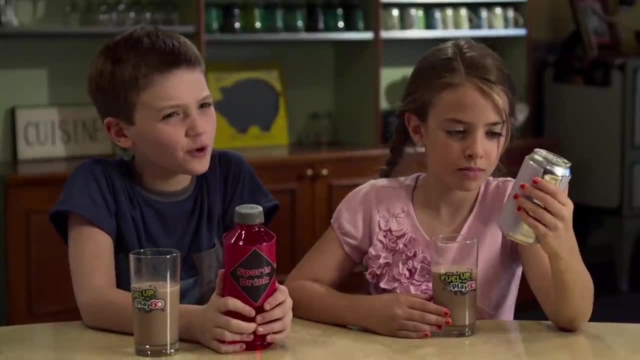 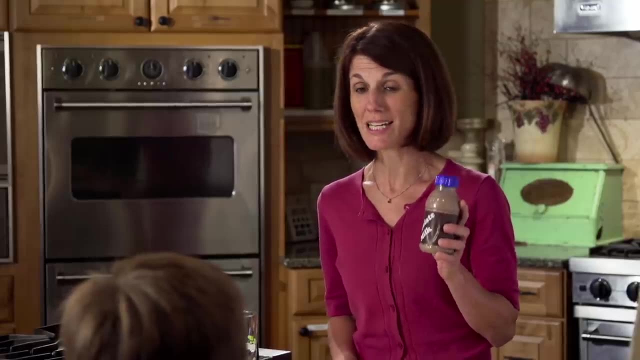 tell me what you see about protein, Mom. there's nothing about protein on this Ava. what about calcium? It doesn't say anything about calcium either. Well, this chocolate milk has protein and calcium, not to mention other nutrients like vitamins A and D and potassium. 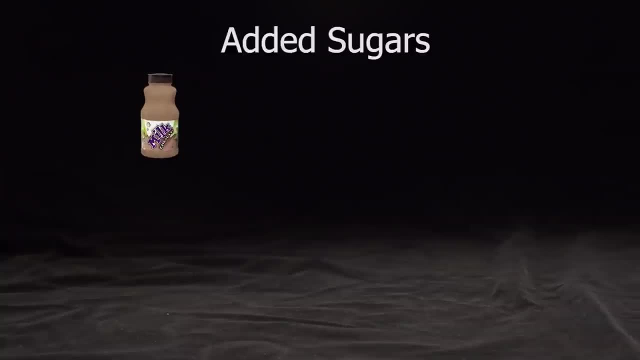 Now let's look at added sugars. Compared to chocolate milk, which has only about 3 teaspoons of added sugar, a bottle of sports drink contains more than 5 teaspoons, And cola, well, it has 8 teaspoons of added sugar. To put that in context, chocolate milk provides the 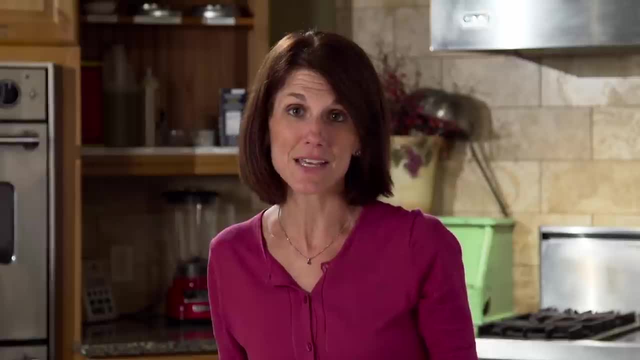 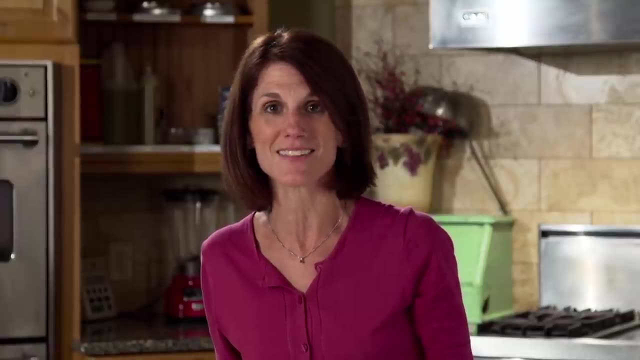 nutrients that kids need for good health, and it has less than half the added sugar of cola. Chocolate milk also helps kids get the three daily servings of dairy that are recommended by the Dietary Guidelines for Americans. When it comes to nutrition, there's no disguising that not all drinks 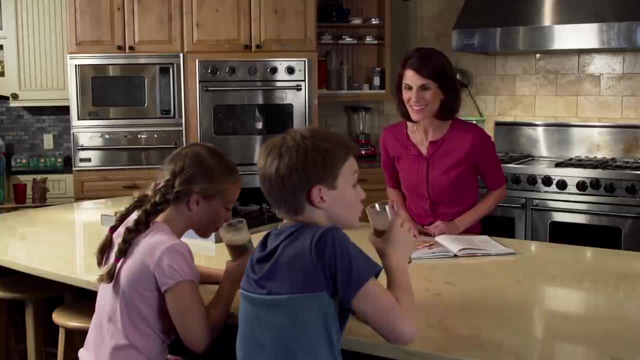 are created equal. Okay, guys drink up. You can find more nutrition information about flavored milk at MidwestDairycom.